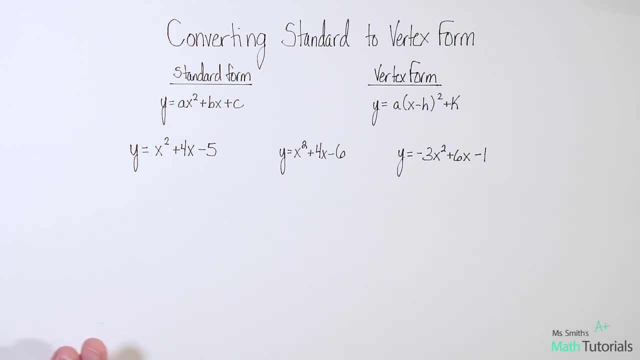 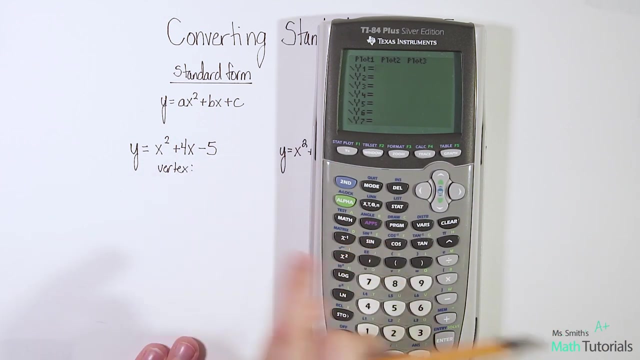 to go from standard to vertex form. I've given you a quadratic here. First thing I need to know is what is the vertex of that quadratic? How can I quickly figure out the vertex on that? Well, we go to y equals and we type in what we've been given. 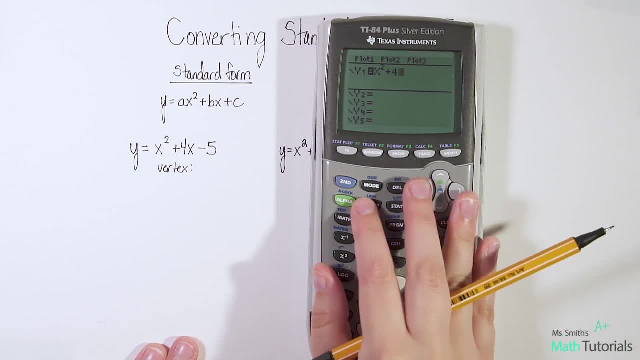 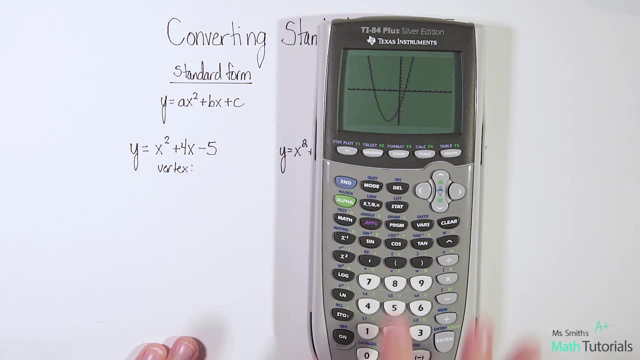 x squared plus four x minus five. okay, I wanna look at the graph picture right there So to find the vertex. I hit second trace and I have to ask myself: is it a minimum or a maximum? So let me look at the picture again. 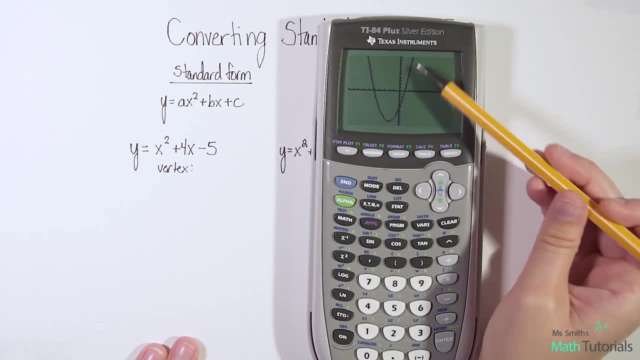 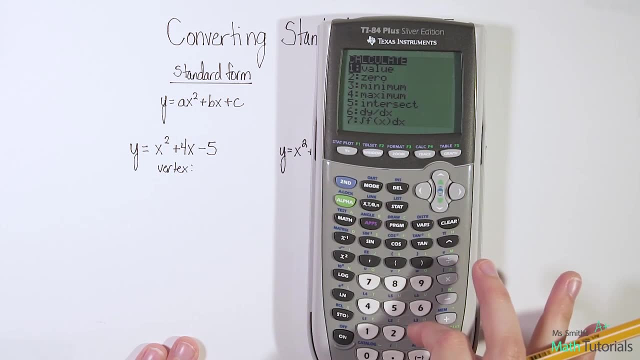 This is at the lower end of the graph. It's a U shape, so that means this is a minimum. okay, We'll look at another one in a minute. that's a maximum. So, second trace, minimum three, and this little blinking spaceship shows up. 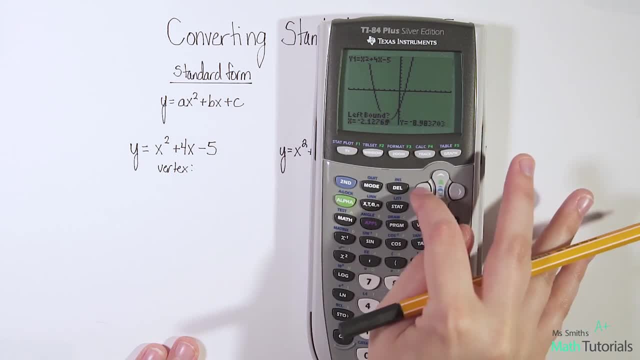 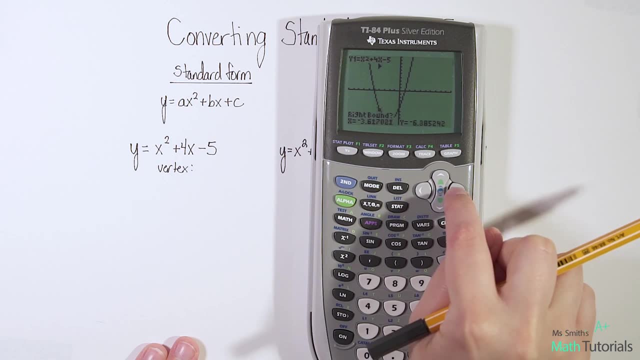 So you want to. it says left bound. So we wanna go a little bit, take it a little bit left of the vertex, So to about right there, lock it in. Now it says right bound. So now we wanna take that and move it. 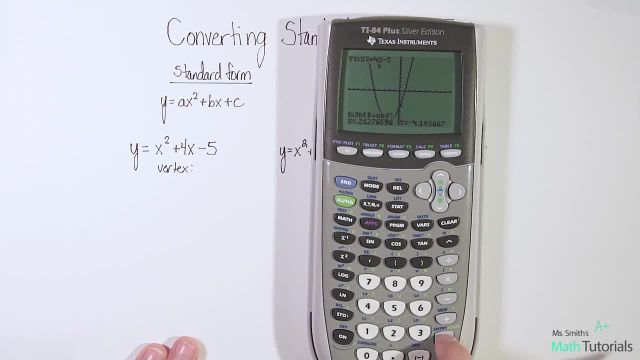 a little bit right of the vertex and lock that in. You'll see those two little triangles show up. as you lock in each side and you hit enter. Okay, so the vertex. here it says negative 1.9.. 9,, 9,, 9,, 9, 9,. we do round that up. 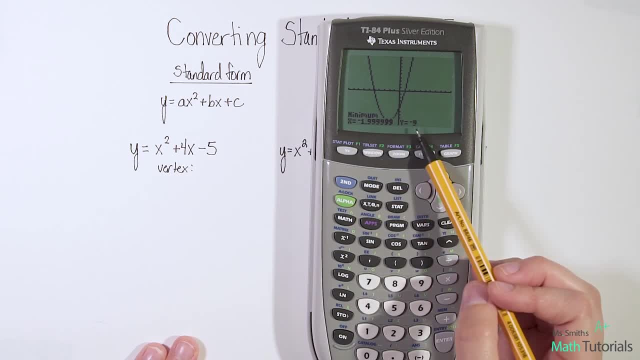 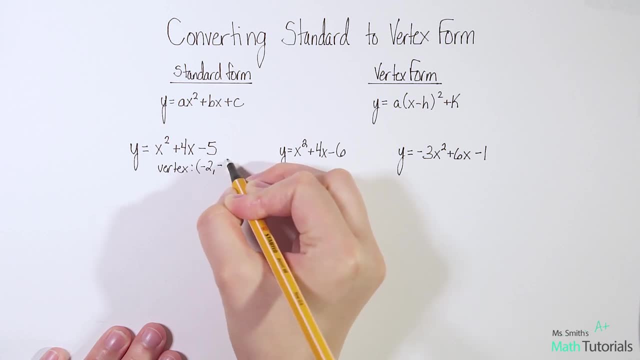 So we would say the vertex is negative 2, negative 9.. So our vertex is negative 2, negative 9.. Once we know that, the rest is really easy. All you have to do is y equals. remember we're creating a vertex form. 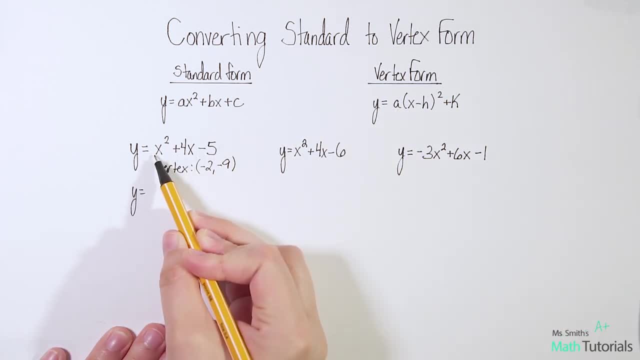 A is whatever the a is in the quadratic, That does not change. So in this case it's just an understood one there. So it's an understood one right for a. Now I have my parentheses x. Now we have our h. 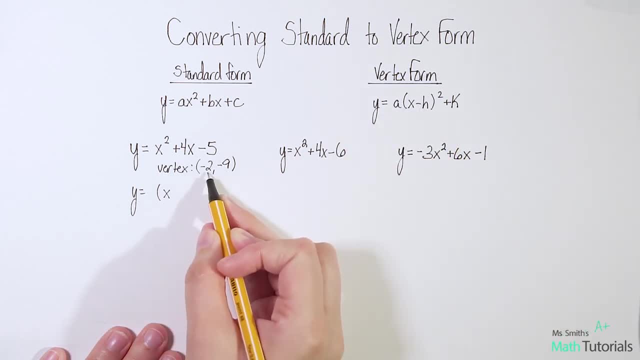 So our h remember is our x value of our vertex. but we flip the sign, So this is minus two. I need to make it plus two, End parentheses squared, and then our plus k. So remember k is our y value. 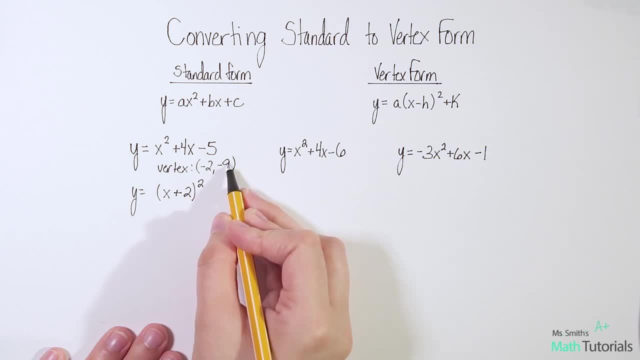 So in this case- and it is the true sign of what we see, So this is negative nine. So I put in minus nine And then you can put the understood one out here. but it's not necessary, You don't need to. 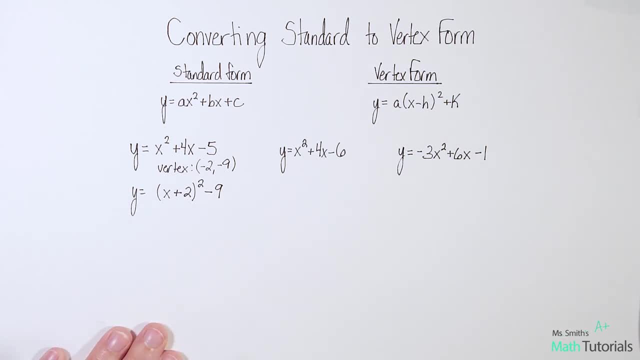 It's understood. So there you go. Quick, simple way to go from standard form to vertex form. All you need to know is the vertex. Let's try another one. For this one we've got x squared plus four, x minus six. 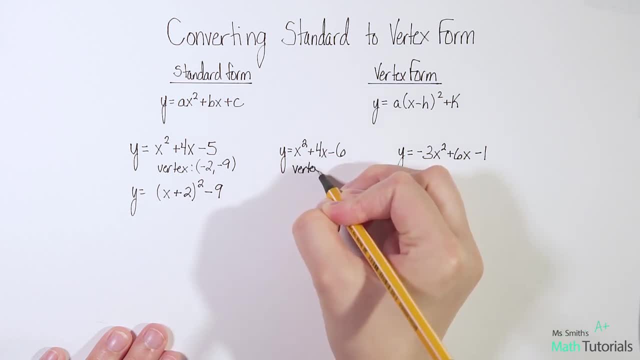 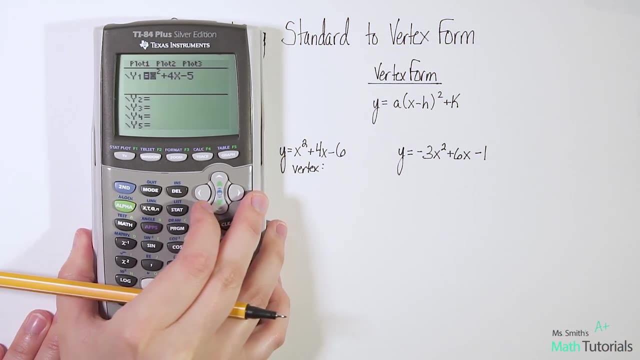 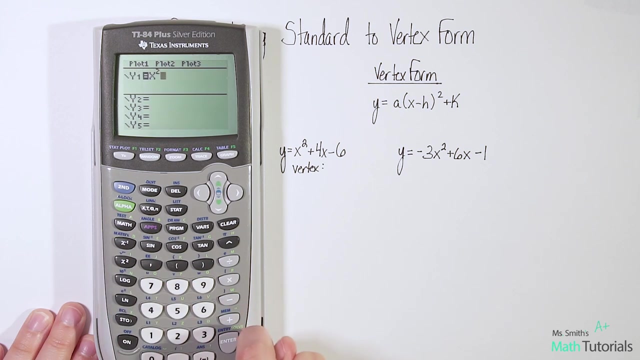 Well, I need to know first what is the vertex. Okay, I'm gonna use my graphing calculator to help me. Go ahead back into your y equals right here, Clear out what we had And let's do x squared plus four, x minus six. 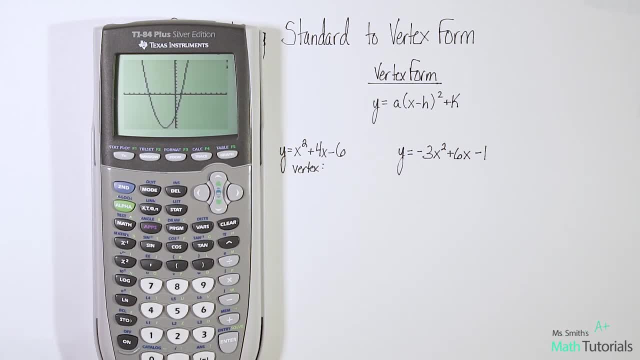 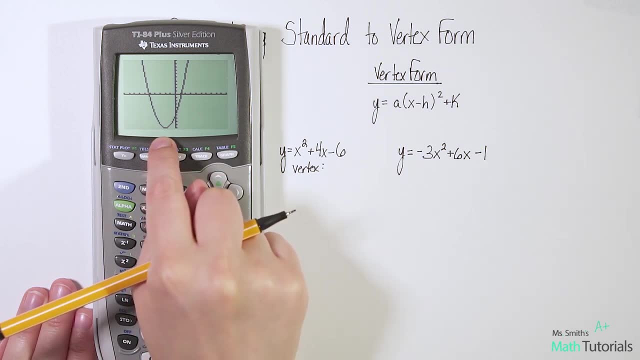 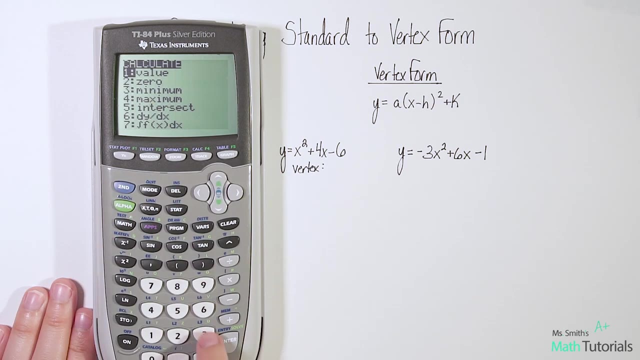 Okay, let's graph it. Let's see how it looks. So note that that is a minimum vertex we are looking for. It is at the lower end of the graph. It's a U shaped. We wanna go to second trace, minimum three. 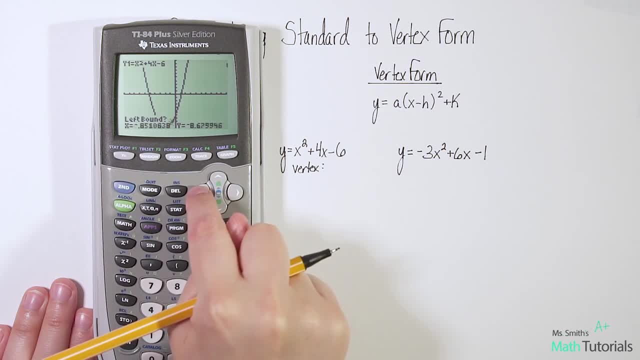 Your little spaceship will show up. We wanna go left bound. first I always put it in center and then move it a little bit left, lock it in back to center and then a little bit right, lock it in and hit enter. 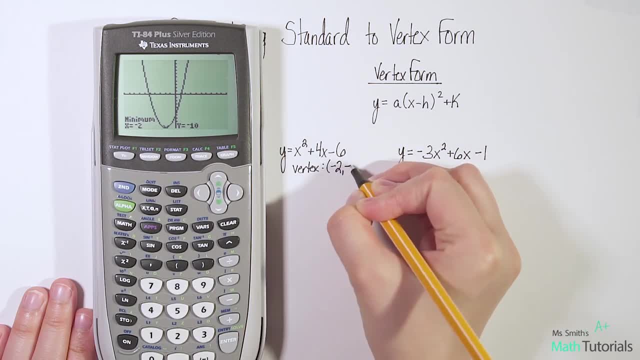 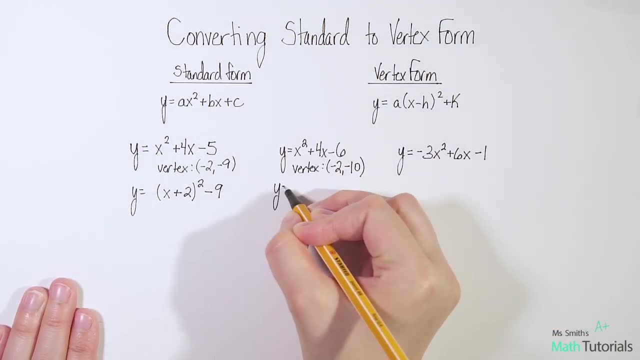 I see my vertex here is negative two negative 10.. So given that information- that's all I need to know- I can now write my standard. my vertex form: quadratic. Remember. a doesn't change, It's whatever a is in the original. 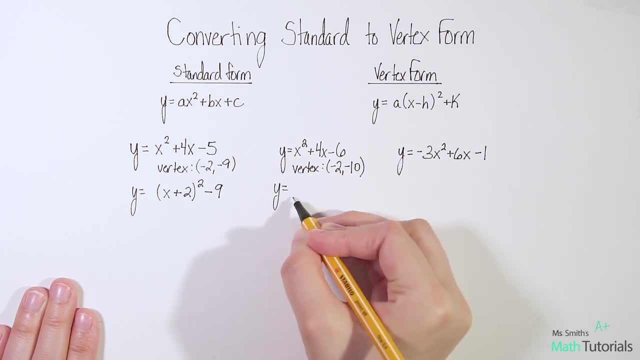 So in this case, again, it's a positive one. I don't need to write a one there, but you can if you wanna see it. Parenthesis x, and then we need our h, So in this case it's a minus two. 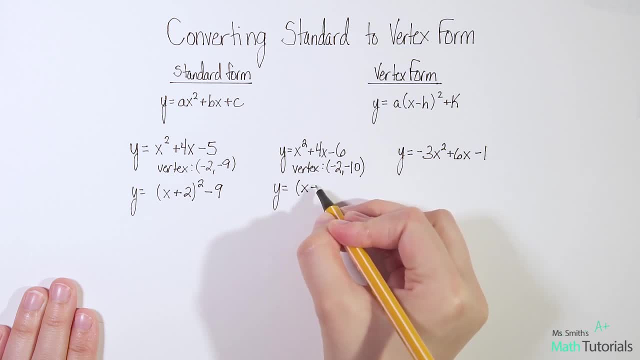 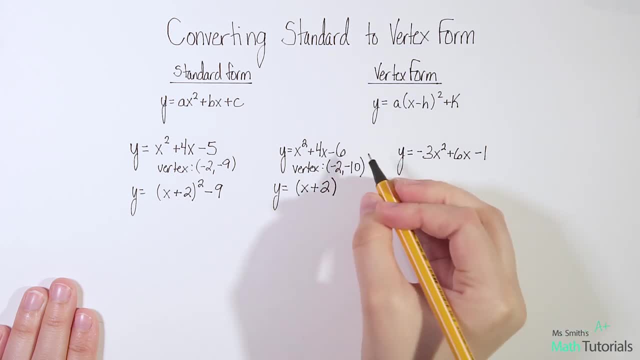 It's the opposite sign of what you're given. It's the opposite sign of what you're given in your vertex: squared and then plus k, squared and then plus k, squared and then plus k. So in this case it'd be minus 10.. 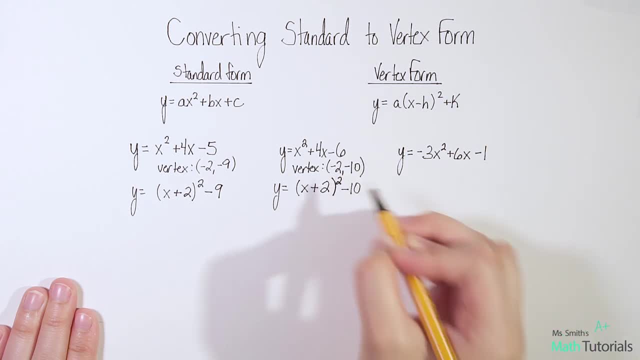 So in this case it'd be minus 10.. The y value is the exact same sign as you are given in the vertex As a quick check, and I should've shown this on number one too, but we can quickly check ourselves to make sure we didn't make any kind of careless error. 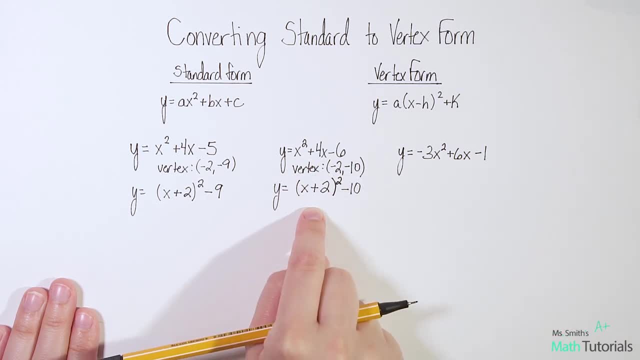 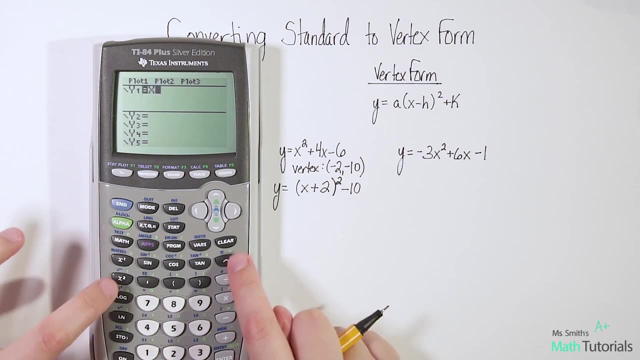 by graphing these two equations. by graphing these two equations, and they should be be the exact same parabola. so let's just double check ourselves. x squared. I'm gonna go to my y equals and type in: x squared plus 4x minus 6, go down to your. 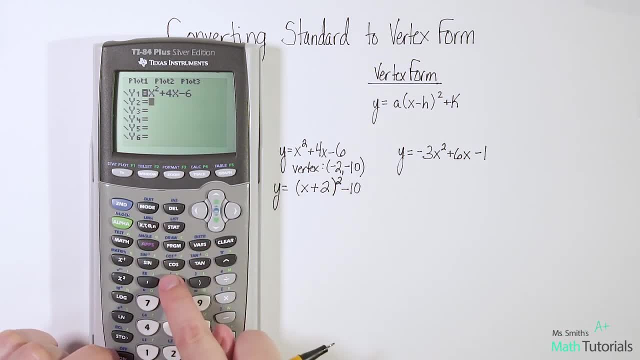 second line and type in the vertex form, parenthesis: x plus 2 squared minus 10. now we're gonna graph it and if we've done it right, it should graph the same line twice. we should not be able to see any difference. okay, see that it's done. 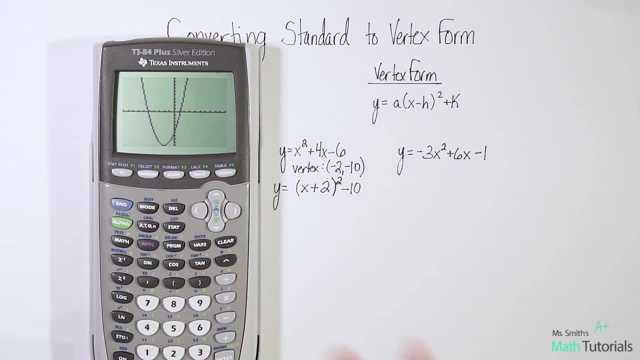 graphing and we have the same line was graphed twice, so that's a way to quickly double check yourself. let's look at this third example. so negative 3x squared plus 6x minus 1. well, first thing we need to know: is the vertex really the only? 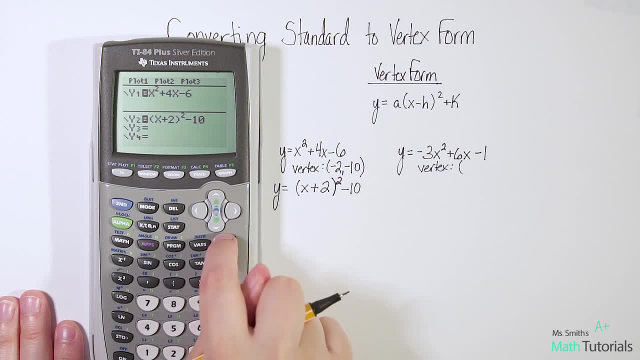 thing we need to know, it's the vertex. so let's go to our y equals. clear out what you need to know is the vertex. so let's go to our y equals. clear out what you had in there: negative 3x squared plus 6x minus 1. let's figure out what is our. 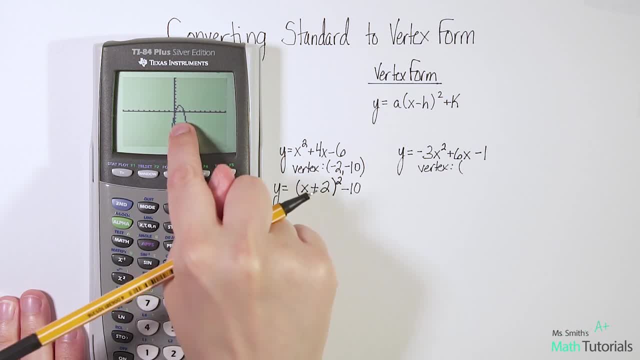 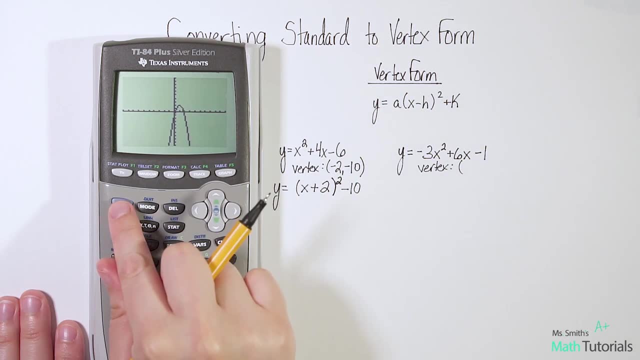 vertex here. notice this time it's a upside down U. that means our vertex is a maximum, not a minimum. this time when we go to second trace we're gonna hit max 4 and notice my spaceship is already a little bit left bound already, so I can go ahead and lock that in. move to the center. move a little bit right bound. 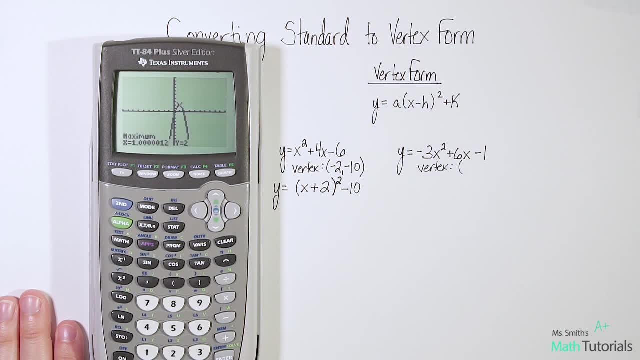 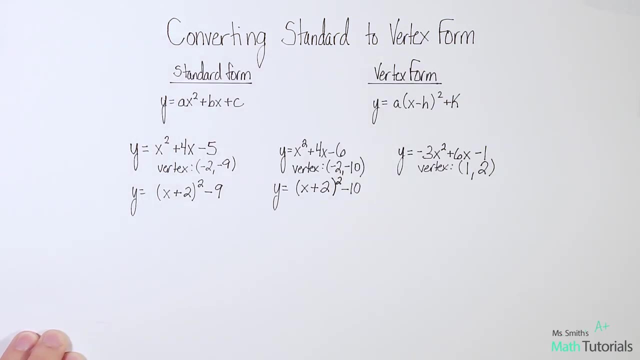 lock that in and then it should tell us our vertex. our vertex follows it now. this says 1.000001.. 1920. we'll just round that to one: positive 1, positive 2. the rest is easy, and just fill it into this form: y equals, remember, a is whatever.